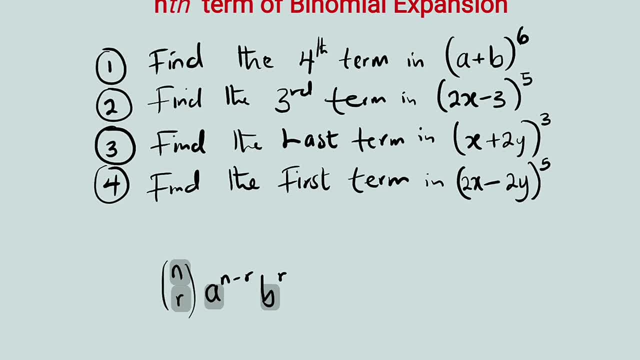 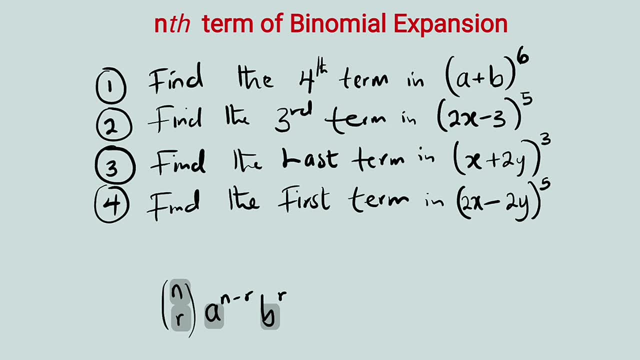 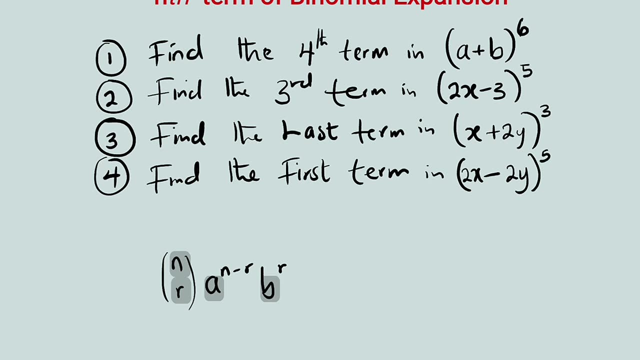 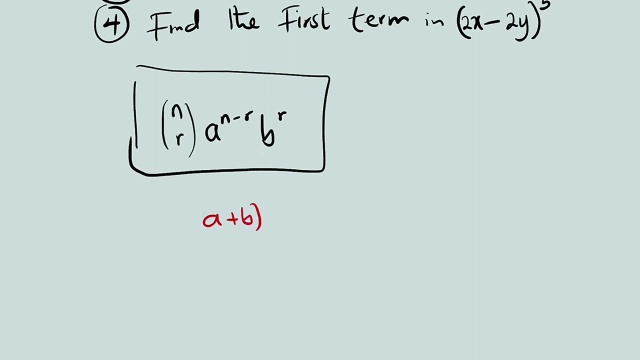 term and b is the second term. So all we have to do in every problem here is to substitute n? r a and b. Okay, let's start with the first one, The first one. we want to find the fourth term in the expression of a plus b to the power of 6.. We have a plus b to the power of 6, which is our first. 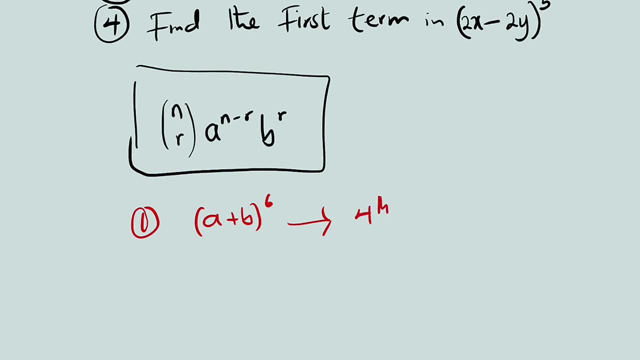 problem and we are looking for the fourth term. One thing you should observe is that in the first term, r is equal to 0.. In the second term, r is equal to 1.. Can you see that r is 1 less than the number of terms. So if you are looking for r, 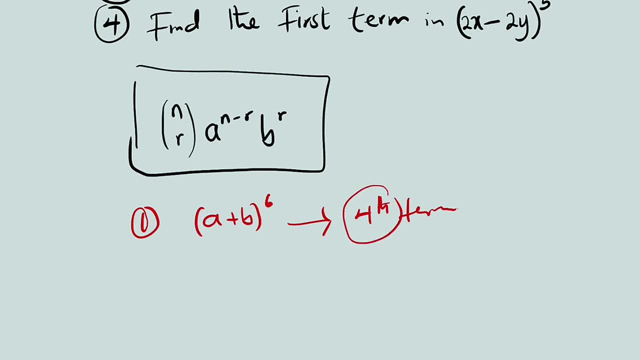 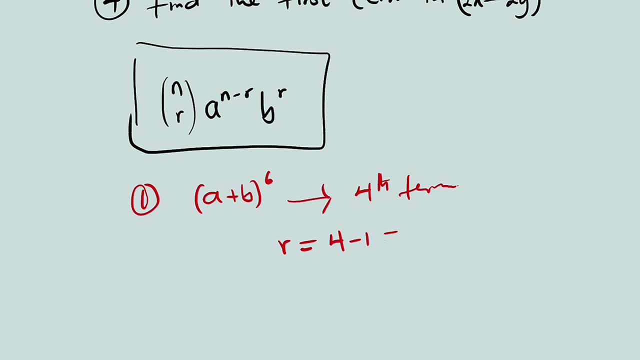 all you have to do is to subtract 1 from 4.. So let's start with r. r is equal to 4 minus 1, which is equal to 3.. n is equal to the highest power, which is 6.. a is a, b is b, so let's substitute. 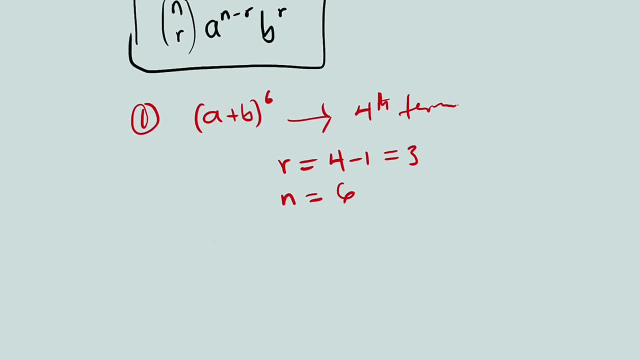 here. Therefore, we have n combination r, which is 3 times the power of 2.. We have n combination. r is 6 combination 3, because r is 3.. Then a raised to the power of n minus r, which is 6 minus 3.. Then b raised to the power of r, which is equal to 3.. Sixth combination r. 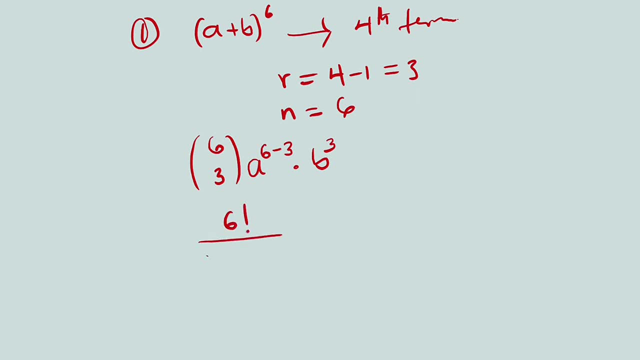 is 6 factorial divided by 6 minus 3 factorial, Then 3 factorial. Then multiply by a to the power of 3, because 6 minus 3 is equal to 3.. Multiply by b to the power of 3.. This is equal. 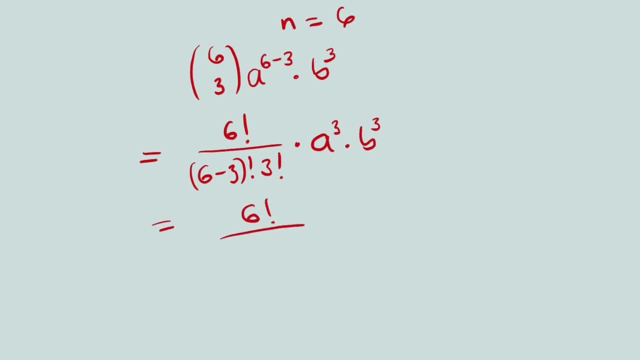 to 6. factorial divided by 6 minus 3 is 3 factorial Multiply by 3 factorial: a cubed, b cubed. Alright, now let us simplify the factorials. This is equal to 6,, 5,, 4,, 3 factorial. I will stop here because I have 3 factorial down. 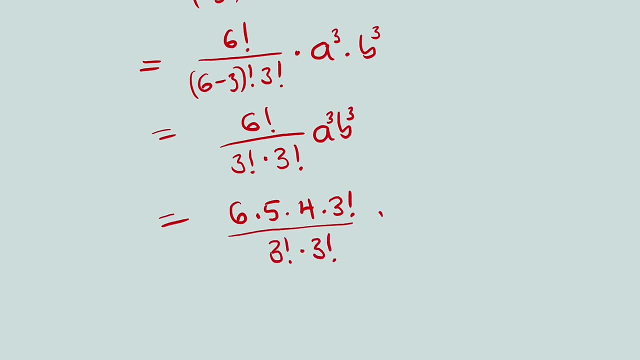 here. So from here, 3 factorial will come out to be 3 factorial. So from here, 3 factorial will come out to be 3 factorial And 3 factorial, remember, is 6.. So let me even break this down: 3 factorial is 3 times 2. 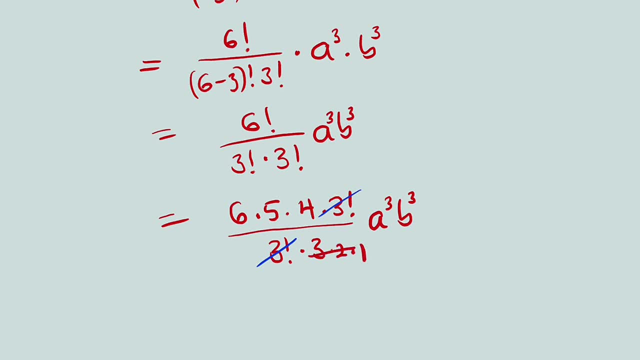 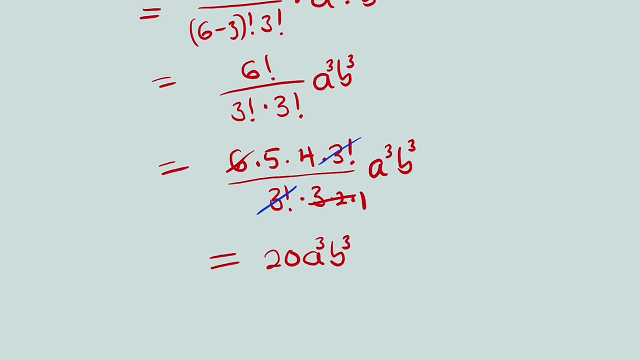 times 1.. 3 times 2 is 6.. So it will cancel this. All we have left is 5 times 4, which is 20.. So finally we have 20. a cubed, b cubed, So this is the fourth term in the expression. 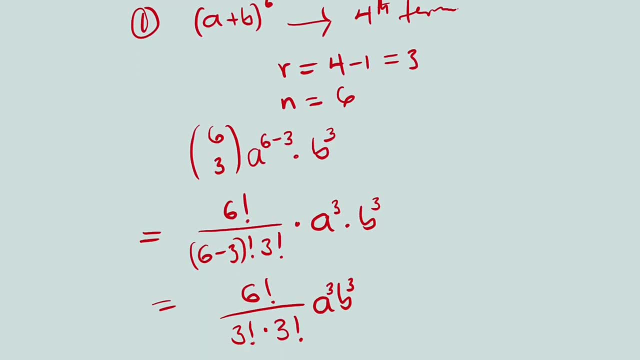 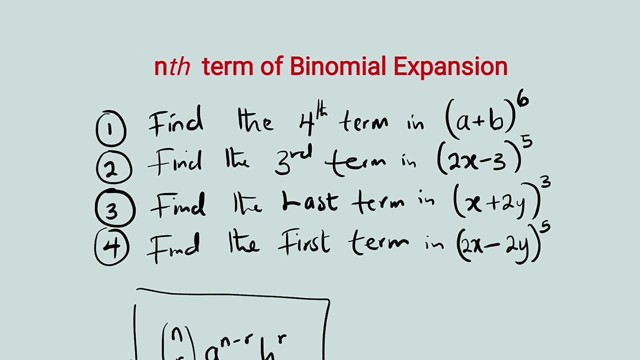 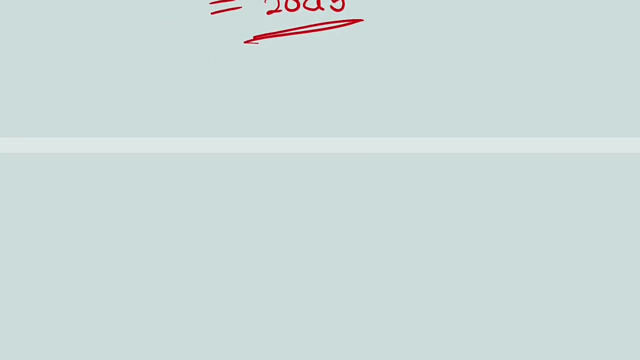 of a plus b to the power of 6.. Now let us take the second problem. The second problem: we have 2x minus 3 to the power of 5, but we are looking for the third term: 2x minus 3. 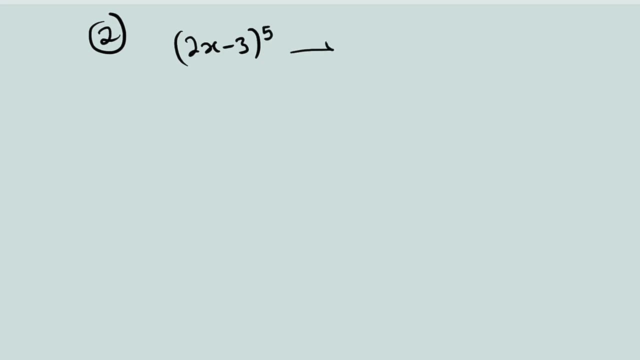 to the power of 5, and we are looking for the third term. Now let me show you what it is: 2x to the power of 5.. The third term is 2 times a cube over a cubed, which is death, a. Now from here you can see that n is equal to 5 and r is equal to 0.. Now let 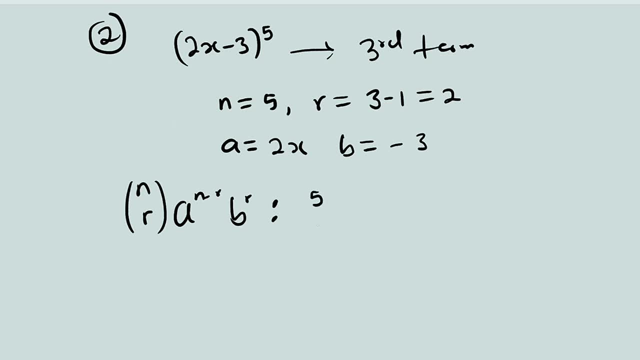 to n is 5. combination, r is 2, then a is 2x. so we have 2x to the power of n minus r, which is 5 minus 2, multiplied by b, and b is negative. 3 to the power of r and r is: 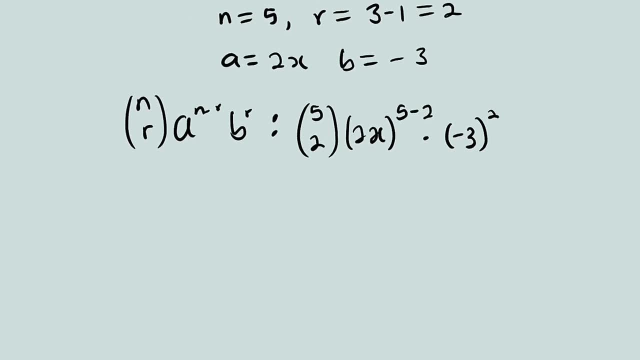 equal to 2. so 5 combination 2 is written as 5 factorial divided by 5 minus 2 factorial, then 2 factorial multiplied by 2x to the power of 5 minus 2, that is, 2x to the power of 3. 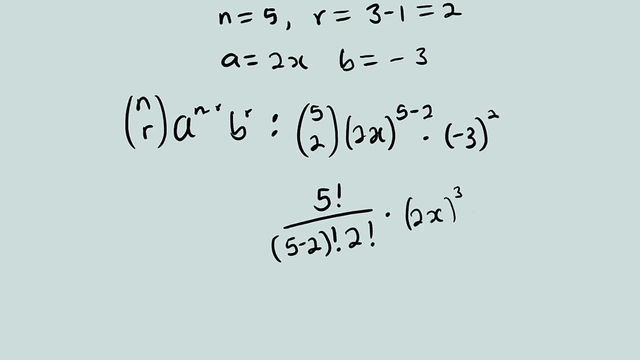 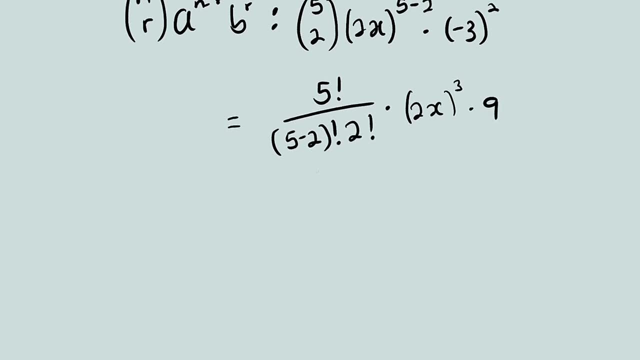 then negative 3 squared is 9. let us further break it down. this is 5 factorial divided by 5 minus 2 is 3 factorial. then 2 factorial multiplied by 2 to the power of 3 is 8. x to the power of 3 is x cubed then. 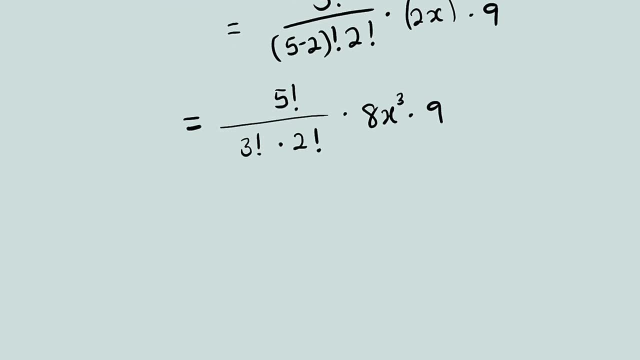 multiplied by 9, 5 factorial is 5. multiplied by 4. multiplied by 9. multiplied by 3. multiplied by. okay, let me stop here, because I have 3 factorial down here we have 3 factorial multiplied by 2 factorial is 2.. so this will cancel this and 2 can go n to 4. 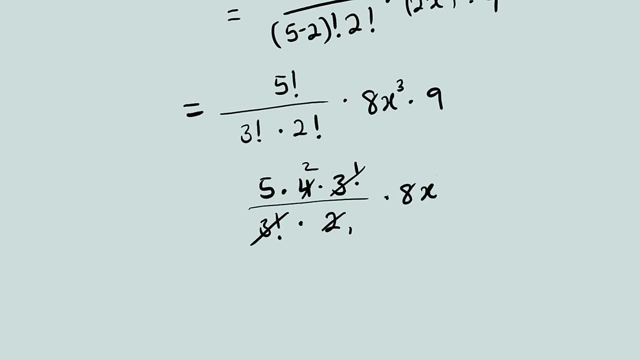 two times. we have times 8x to the power of 3 times 9.. so 5 times 2, here is 10.. so this is 10 multiplied by 8x, cubed times 9.. so let us multiply 10 times 8 times 9.. 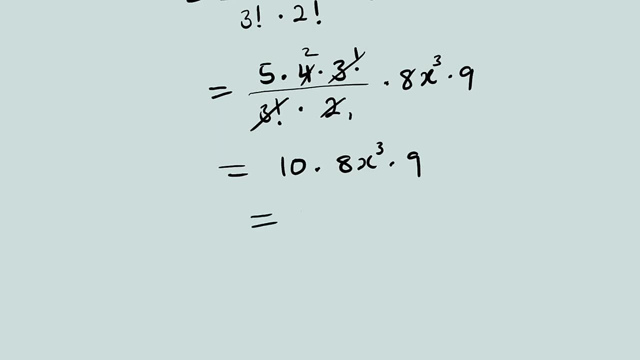 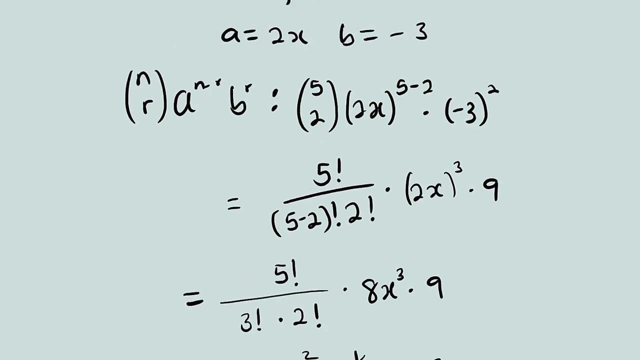 10 times 8 times 9 is 720. so we have 720 x to the power of 3.. so this is the third term in the expansion of 2x minus 3 to the power of 5.. let us take problem number 3. 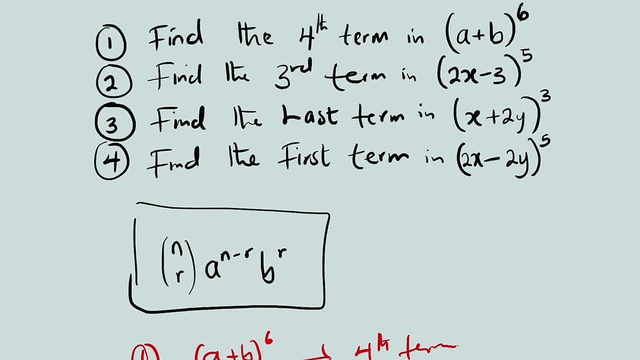 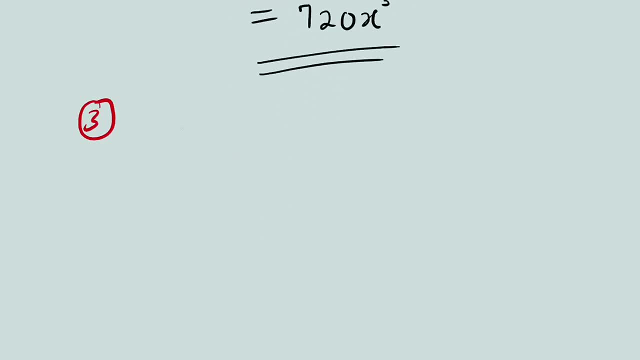 problem number 3: we are looking for the last term In the expression of x plus 2y to the power of 3.. x plus 2y to the power of 3.. And we are looking for the last term, So let's write the data. 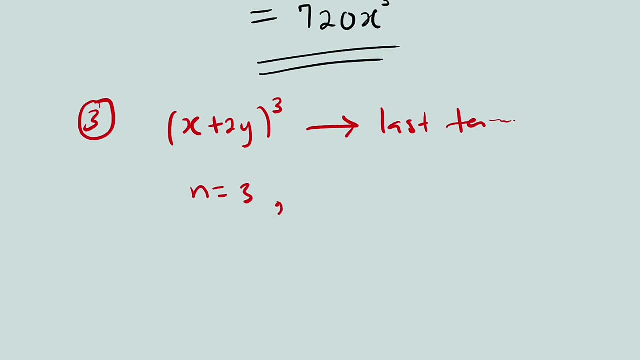 n is equal to 3 here, Then which one? r is equal to 3 as well, Because in the last term r is equal to n. That's what you should know. Then a is x, b is 2y. 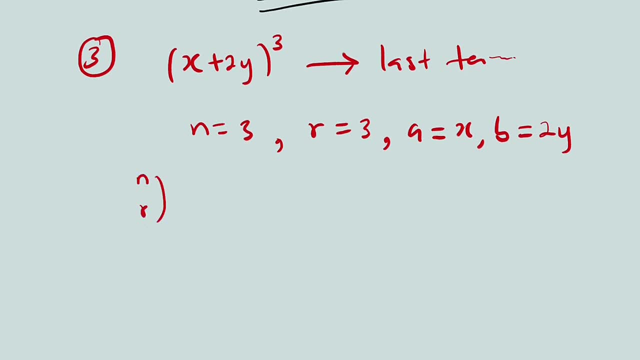 Then for the formula, it remains n combination r, a raised to the power of n minus r, b raised to the power of r, And this is equal to n, is 3.. Combination 3, again Then a, which is x to the power of n minus r. 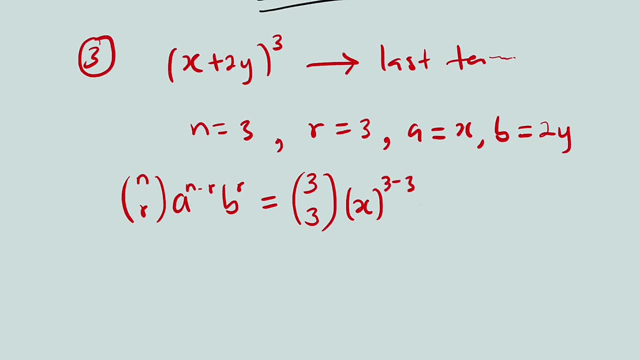 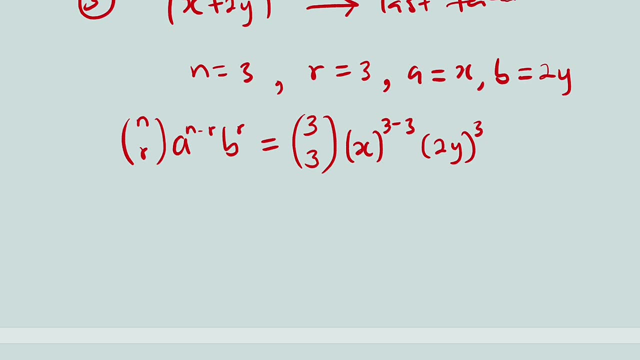 That is 3 minus 3.. Then b, which is 2y raised to the power of r, And r is 3.. Remember that n combination n is equal to 1.. Therefore, 3 combination 3 is equal to 1.. 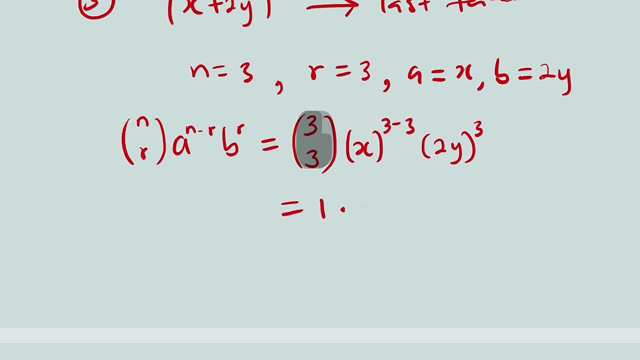 So we have 1 multiplied by x to the power of 0. Because 3 minus 3 is 0. Then multiplied by 2y to the power of 3, is 8y cubed, This is 1, because x to the power of 0 is 1.. 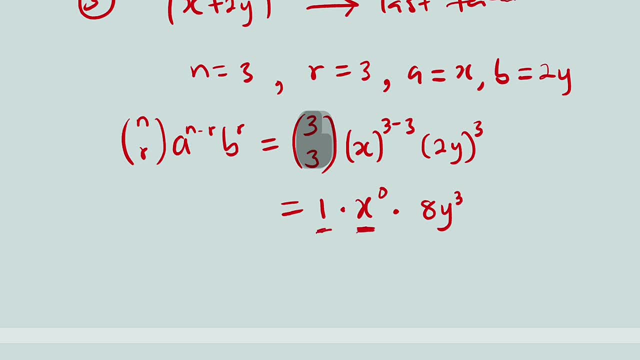 So we have 1 times 1 times 8y to the power of 3.. Finally, we have just 8y to the power of 3 as our last term After expanding x plus 2y to the power of 3.. 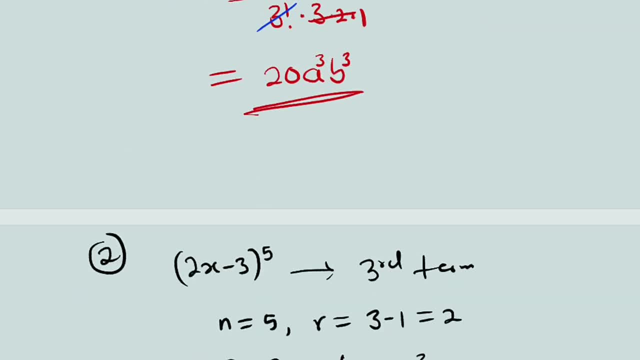 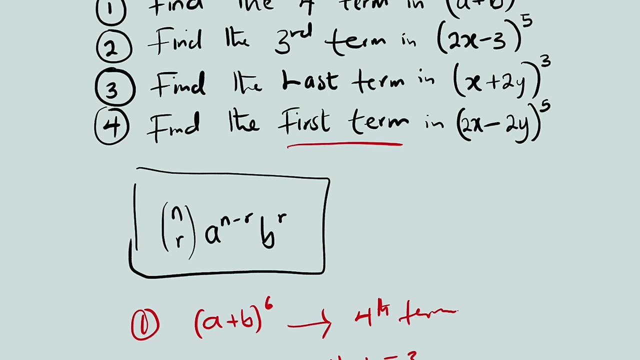 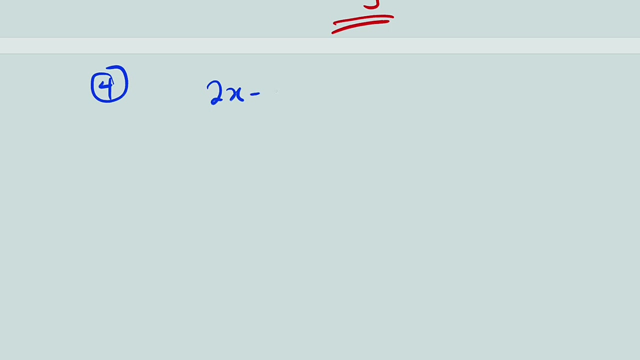 Now let us take the last problem. The last problem: we want to find the first term in the expression of 2x minus 2y to the power of 5.. 2x minus 2y to the power of 5.. 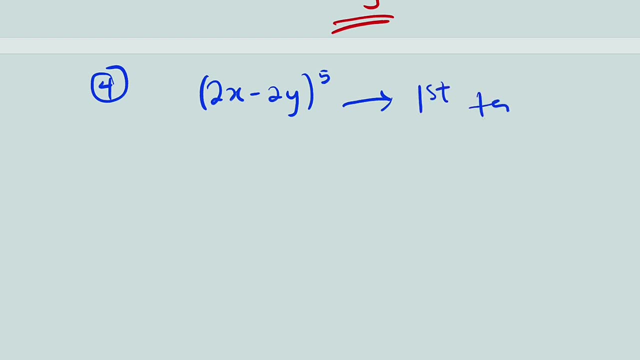 We are looking for the first term. Remember, in the first term r is 0.. So n is 0. So n is 5.. r is 0.. a is 2x, Then b is negative 2y. Therefore we have n combination r. 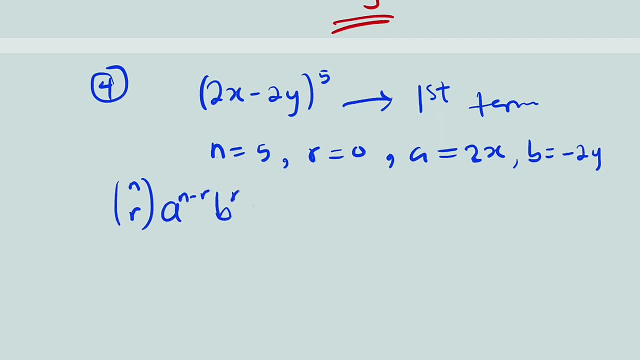 a raised to the power of n minus r. b raised to the power of r, which is equal to n, is 5 combination 0.. a, which is 2x raised to the power of n minus r, that is 5 minus 0..